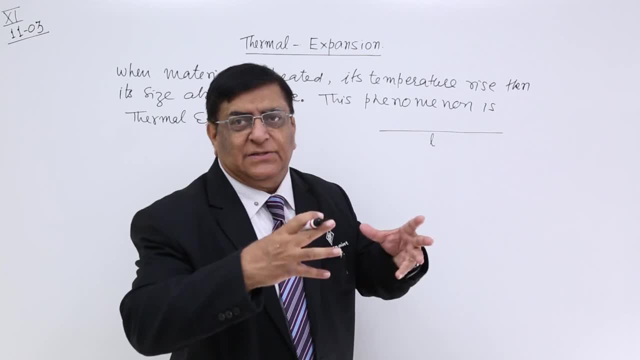 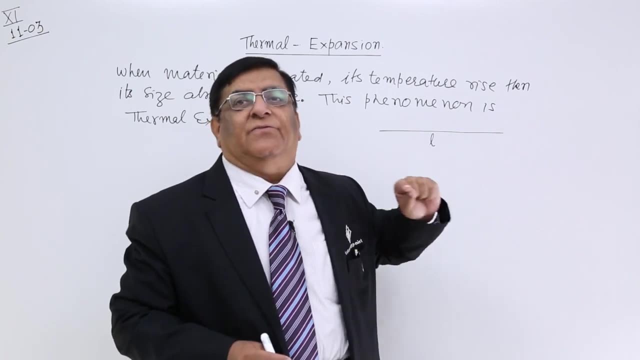 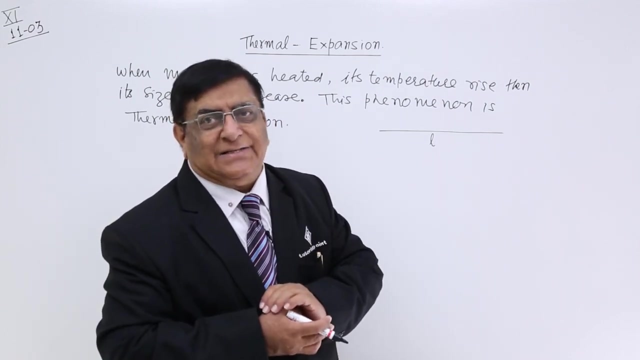 When we heat it, it expands in all directions, but the width increase and the depth increases so small that we neither can measure it and we would not like to measure it. we just neglect it. In that case, what we observe, and what is significant, is increase in the length. 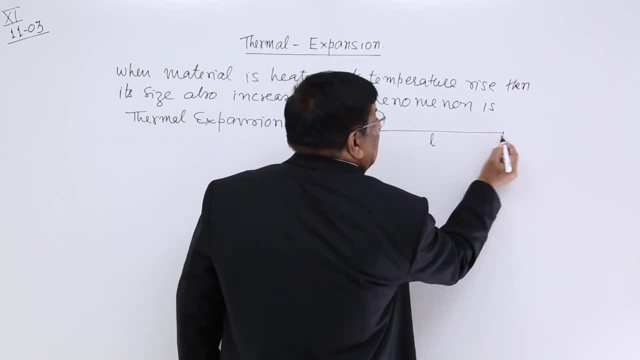 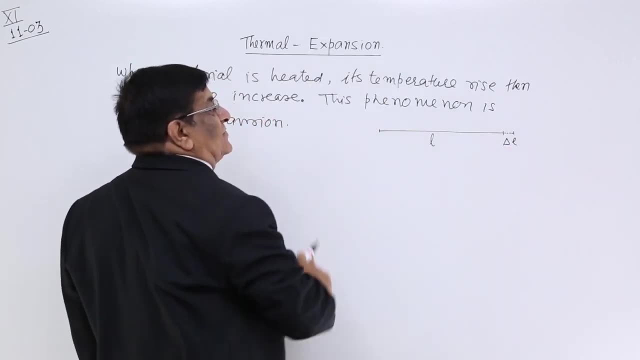 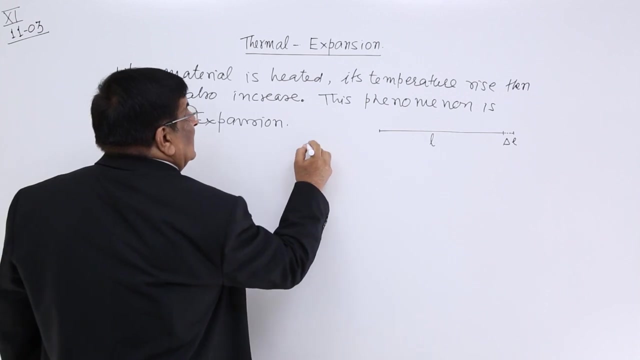 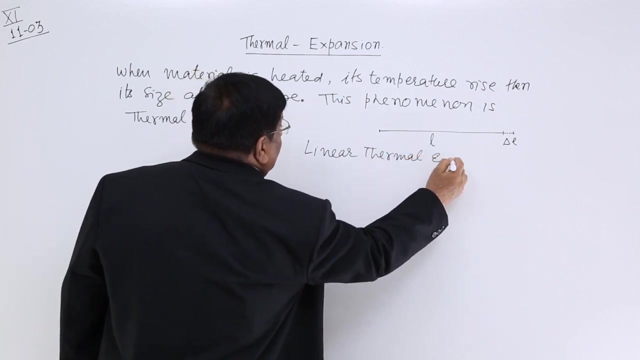 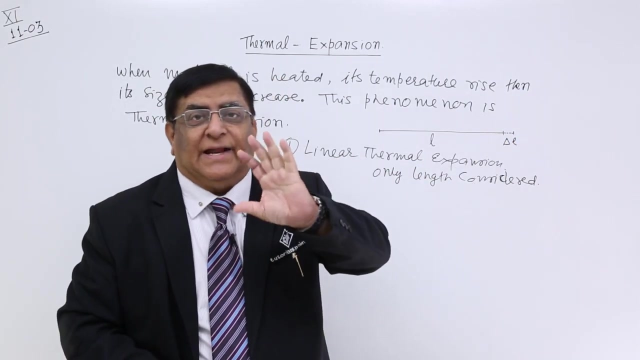 and when we heat it, its length increase by a certain length. This is expansion, thermal expansion. because this thermal expansion is in one line, we call it linear expansion, Linear thermal expansion. Please do not think that only length is increasing. width and depth are not increasing. 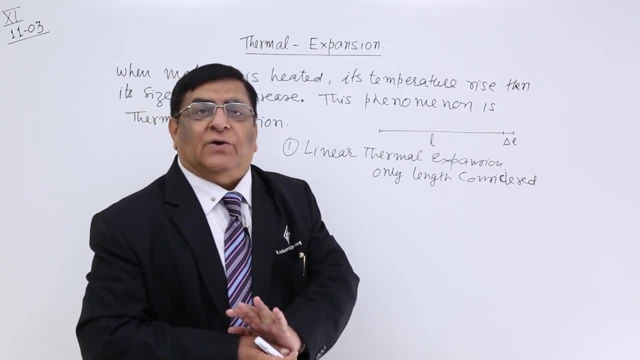 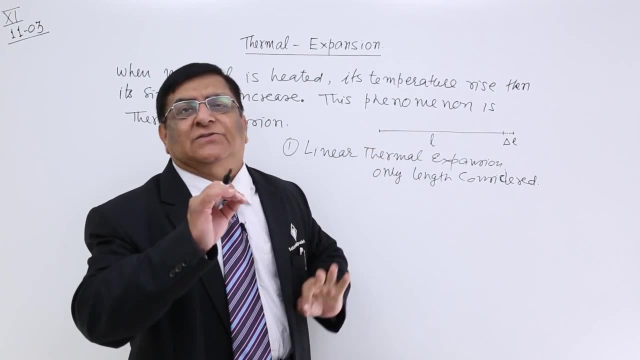 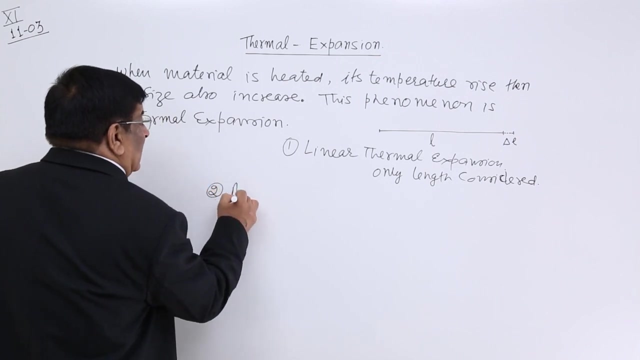 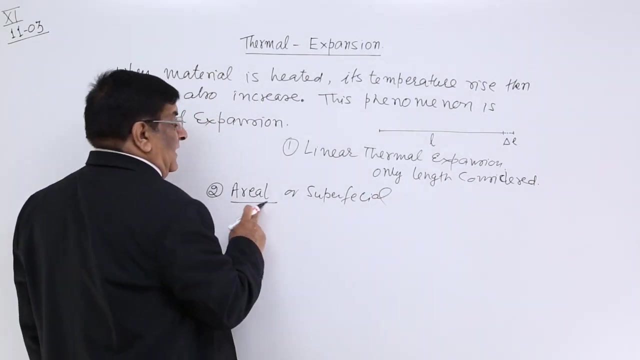 Everything is increasing. but when we go, which can be neglected one, width and depth are very small, their increase is almost zero, So we neglect it. This is thermal expansion. Second is areal or superficial Areal regarding area, This is a plate. 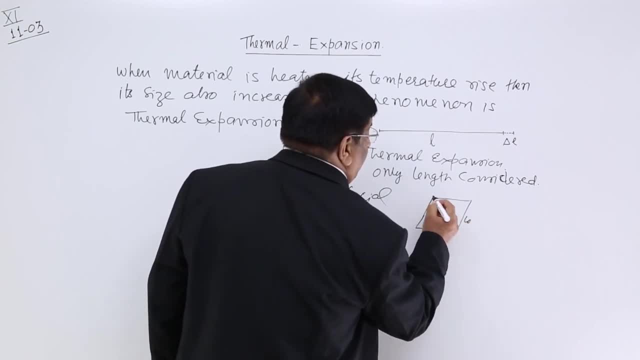 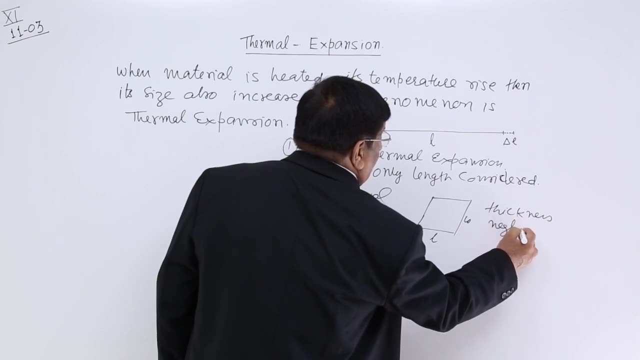 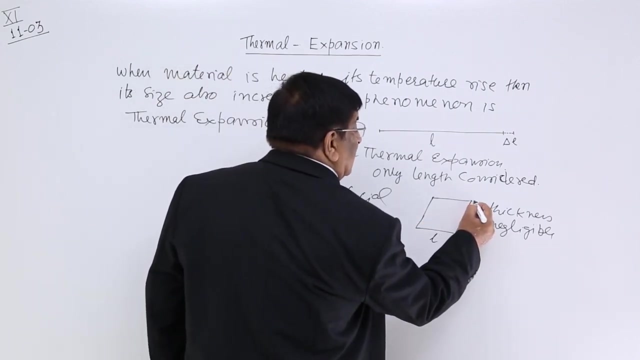 which has got length, which has got width, but thickness is negligible. So when this is heated up, the temperature is given to it. we find the length has increased, the width has increased and we get the new area like this: The length has increased, the width has increased. 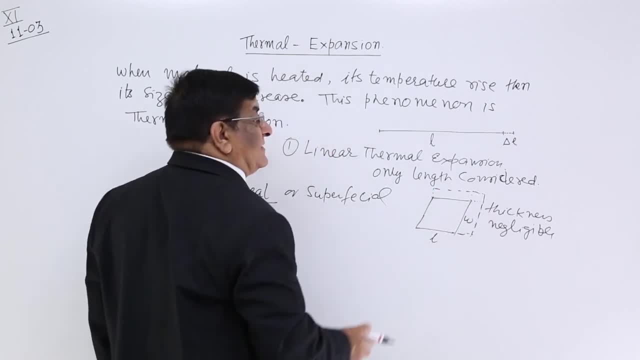 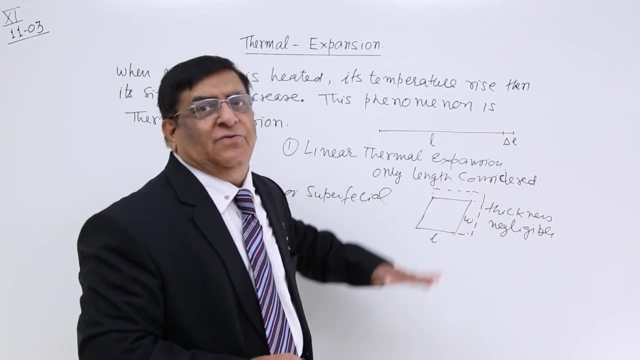 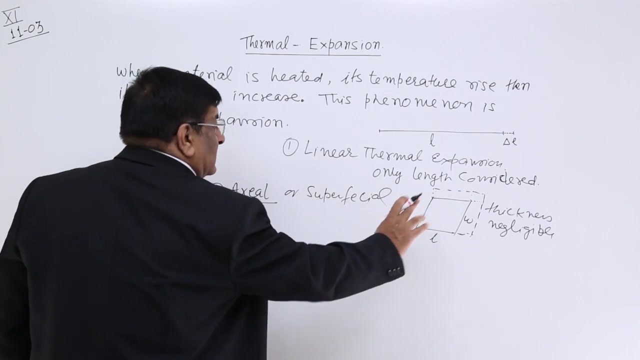 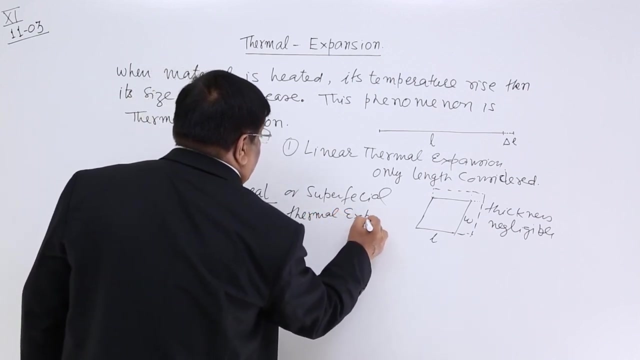 And therefore the total area has increased, and this increase is significant. The depth is neglected. There is an increase in the depth. we neglect it When we are considering this case. we say it is areal or surface Superficial thermal expansion.